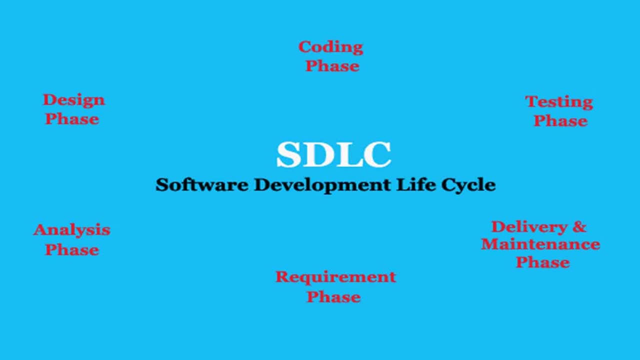 Second one: Analysis. Third one, Design. Fourth one: Coding or development. Fifth one: Testing. Last one: Deployment and maintenance. Next, one important note. It is general software development life cycle. We have various SDLC models in the IT industry: Waterfall model, V-model, Spiral model and famous Agile development models, etc. 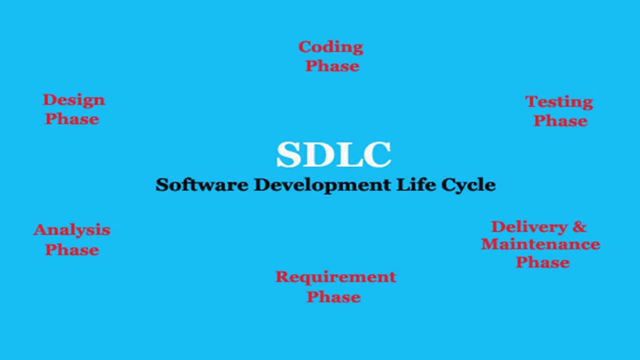 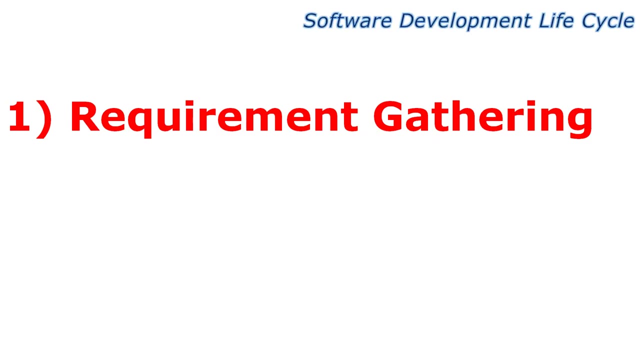 Software development process varies from one SDLC model to another. Next First phase in this life cycle: Requirements gathering. Requirement gathering is the most important phase in SDLC software development life cycle. Business analyst collects the requirements from the customer or client as per the client business needs. 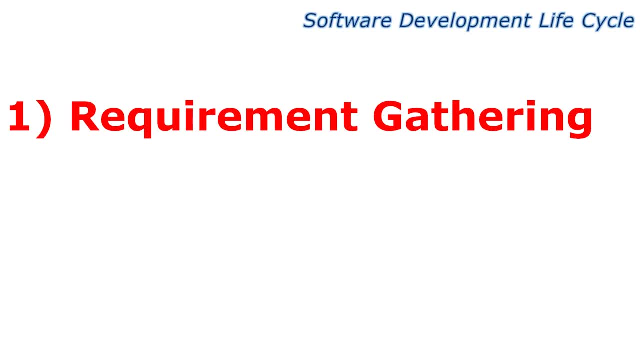 And documents the requirements in the business requirements specification BRS And provides the same to development team. One small note: Document name may vary from one organization to another. Some examples are Customer requirements specification CRS, Business requirements document, BRD, etc. Next phase in this life cycle. 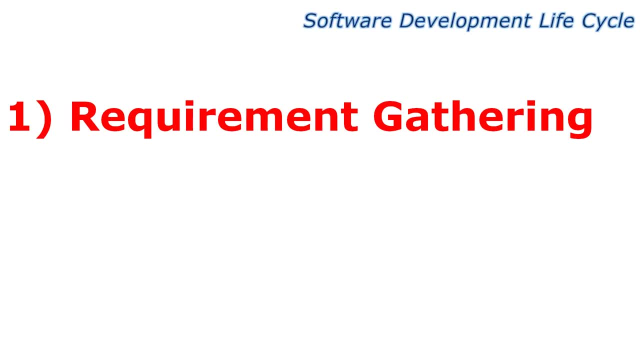 Next, another criteria: Suppose our planned software is not only for single customer and the software product for multiple customers. Then business analyst or business team collects requirements from the market and also evaluate other similar products in the market. Next, Key role in this phase is and Business analyst. 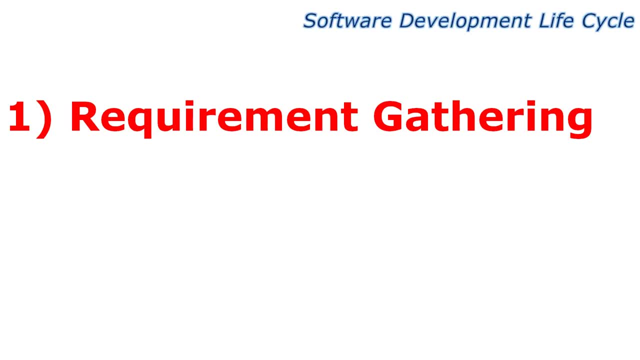 and sergeant, and business requirement classification such as RAẻ. Next Analysis: Once the requirement gathering is done, The next steps is to define and document the product requirement and get the upload by the customer through SRS software requirement specification. SRS consists of all the product requirements. 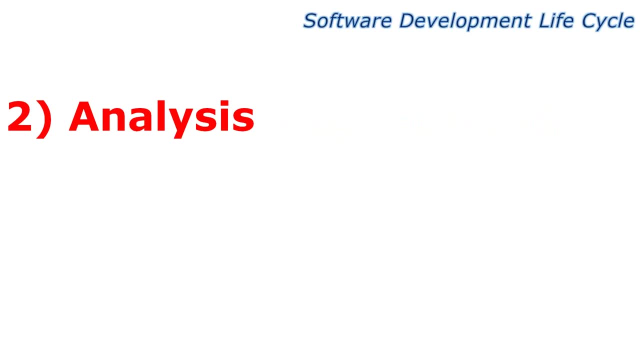 to be designed and developed during the project life cycle. Next, key people involved in this phase are project manager, business analyst and senior members of the team. The outcome of this phase is software requirement specification, SRS. Next design In design phase, senior. 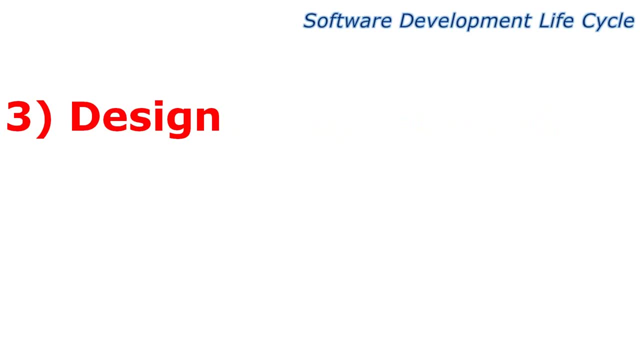 developers and architects. they give the architecture of the software product to be developed. It has two important steps. One is HLD- high level design, or global design, And another is LLD- low level design, or detailed design. HLD- high level design is the overall 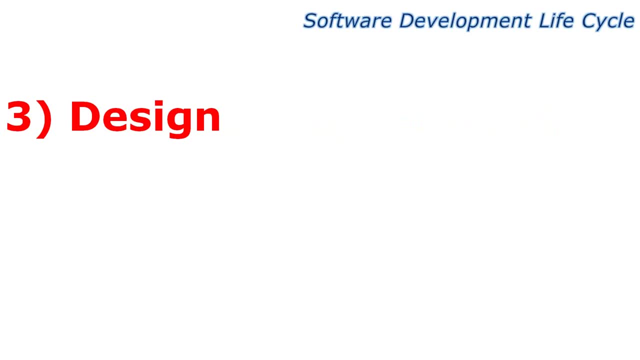 system design covers the system architecture and database design. It describes the relation between various modules and functions of the system. Next low level design: LLD. This is the detailed system design covers how each and every feature in the product, how, 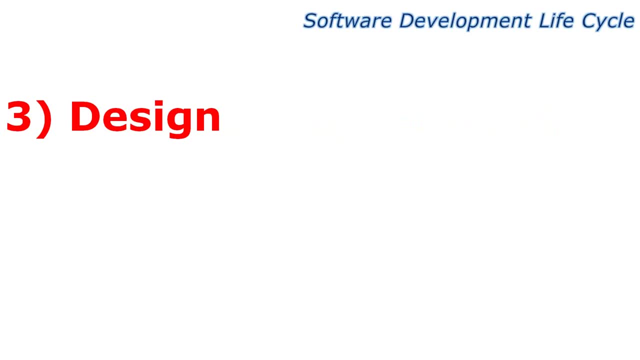 every component should work Next. the outcome of this phase is high level design document and a low level design document, Design documents. This document works as an input for next stage: coding, next coding or development, or you can say implementation developers- senior developers, juniors, fresher- also involved in this phase. this is the phase where we start building the software. 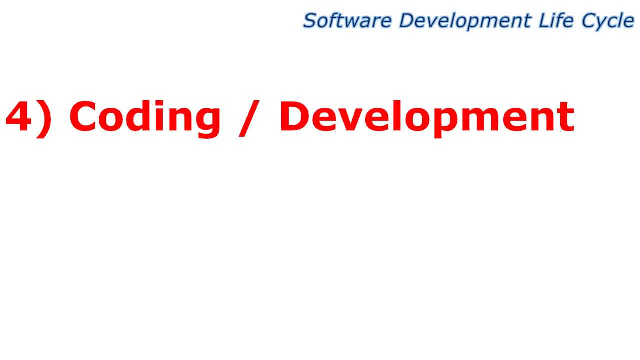 and start writing the code for the product. the outcome of this phase is source code document and the developed product. next important phase: testing. once the software is complete, then it is deployed in the testing environment. the testing team starts testing. either test the software manually or using automated test tools depends on process defined in stlc.